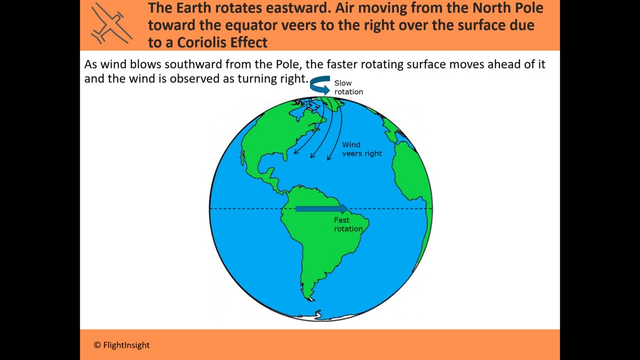 What that's going to do is, as there's an initiation of a flow of air, for example, from the North Pole southwards, rather than moving in a straight line, that straight line, as it moves further and further down, is going to be left behind by the turning Earth. 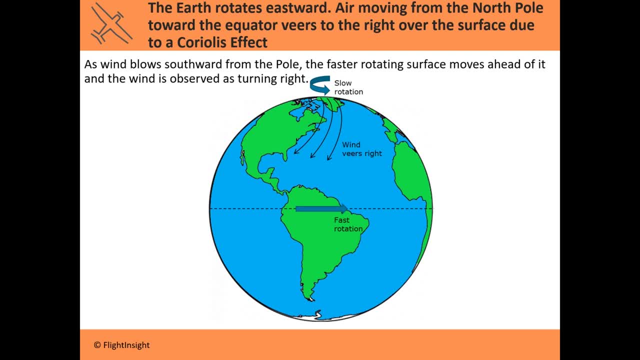 So as the world moves to the east, or as it moves counterclockwise like that, it's moving in front of that moving Earth. So it's going to appear as if that wind is veering to the right. The faster rotating surface moves it ahead, or the surface moves ahead as the wind blows behind it. 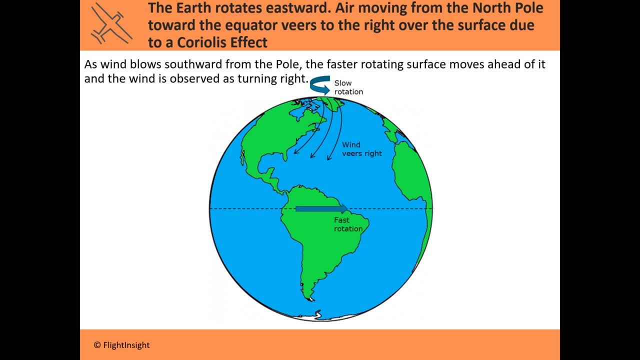 So any wind that's initiated is going to have a rightward veer to it in the Northern Hemisphere and a leftward veer to it in the Southern Hemisphere. We're going to forget about the Southern Hemisphere. This is the FAA private pilot. We're in the United States, so we don't have to feel too bad about leaving. 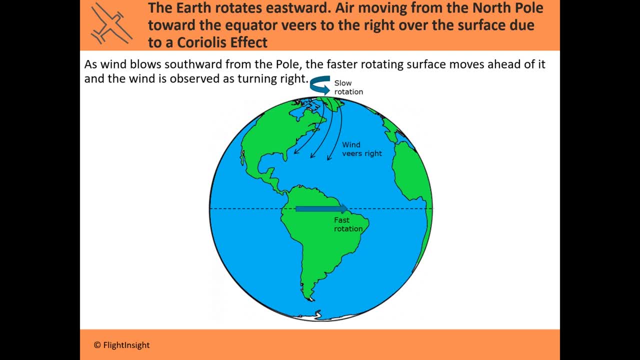 out our friends in the Southern Hemisphere when we only talk about the effects of Coriolis effect and things like that from the perspective of us in the Northern Hemisphere. So we'll keep it simple for the rest of the course and only talk about wind veering to the right as the initiating pressure gradient is deflected by the Coriolis effect. 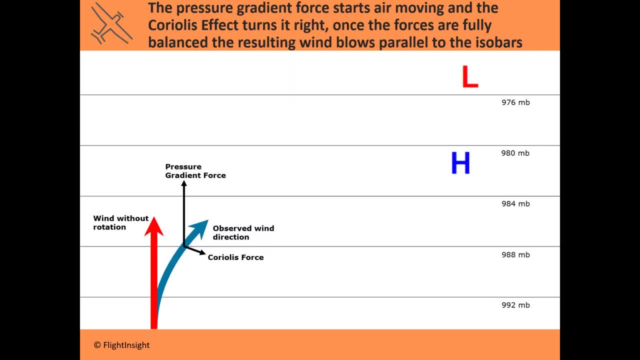 What it boils down to is that you have two forces that are causing the wind to blow. You have an initiating force, That's the pressure gradient force that Starts the air moving from high to low, and we can think of that as moving perpendicular to isobar. 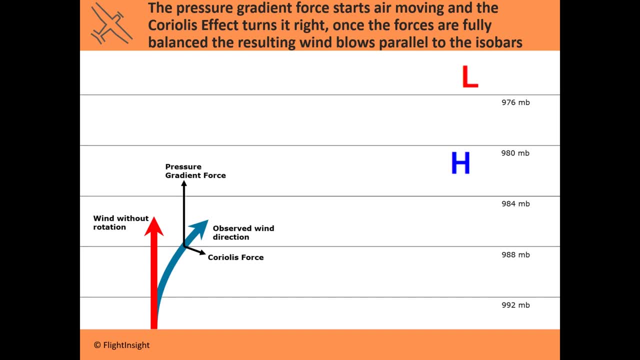 So you see, the five isobars that we have spaced here is horizontal lines and that red arrow that's moving perpendicular to it, That's not being affected by the Coriolis. That's that initiating force, But then a Coriolis effect is going to deflect it to the right and that's that blue arrow there. 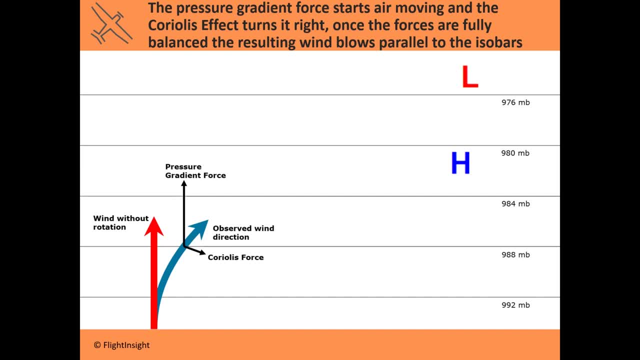 So as that takes effect, you notice that the perceived wind direction is going to veer to the right. So that's the blue arrow there off to the right of what the pure pressure gradient force looks like. So now, as this continues, we can see the effect that Coriolis has as that wind 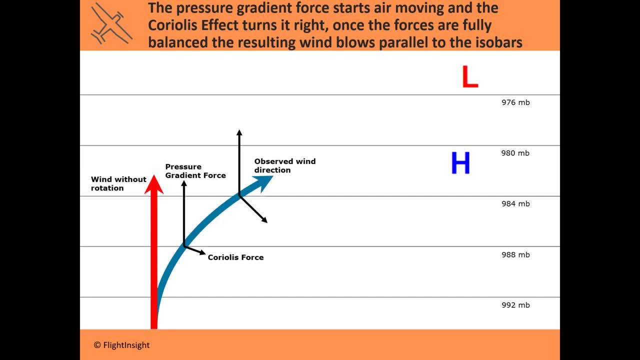 continues on, And so, once Coriolis has taken its full effect, it's taken that wind that was initially moving across the isobars and it's now causing it to seem to move parallel with the isobars And notice the phenomenon right Pressure gradient. 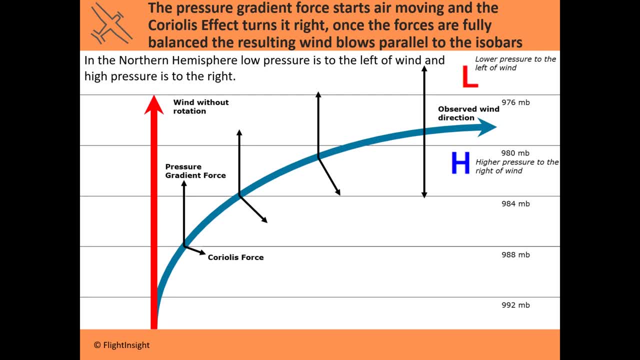 force is now being counterbalanced by Coriolis force, And when those two forces are in direct opposition, you have the observed wind direction flowing parallel to those isobars. Notice another thing here: Because it's veering to the right as it moves from high to low, it's causing the wind to have the high pressure. 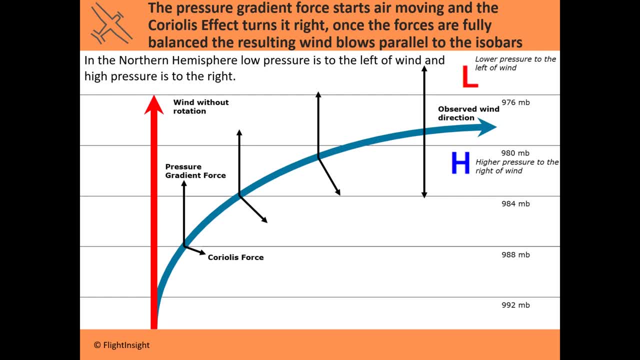 system or the high pressure air to the right of it and the low pressure system of air to the left of it. That's going to be really important in determining the direction of airflow in a low pressure system and a high pressure system. You can see kind of where we're getting at If you have a high pressure system. it 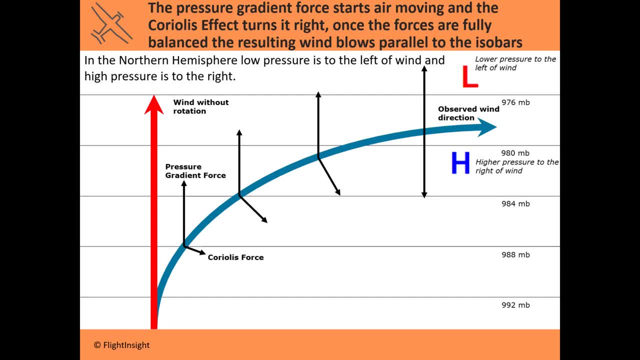 means that the wind is always going to be blowing to that side of it. that makes the high pressure on its right. As you get closer and closer and closer to the high pressure system, you're observing the wind off to that side. Same thing on the low pressure. So we'll see how that. 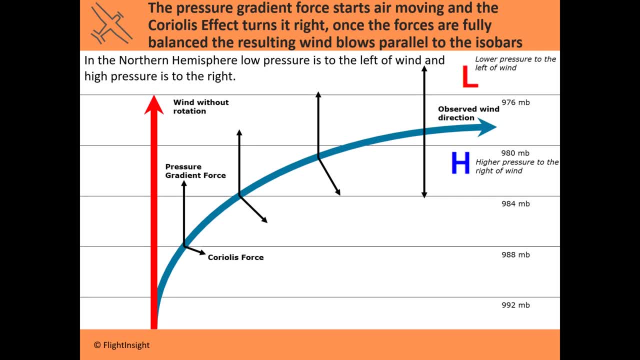 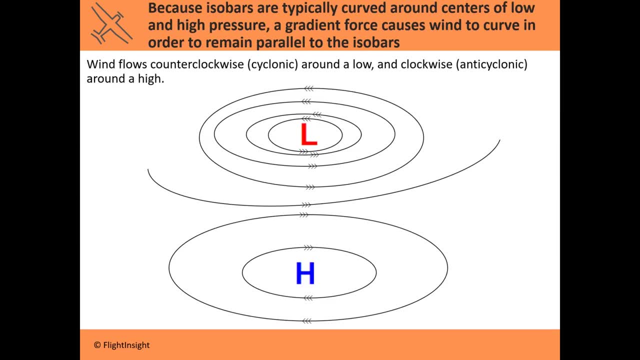 kind of plays out when we create these systems. But in the Northern Hemisphere the high pressure is to the right of the wind and the low pressure is to the left of the wind, So keeping that model of low pressure to the left of wind high. 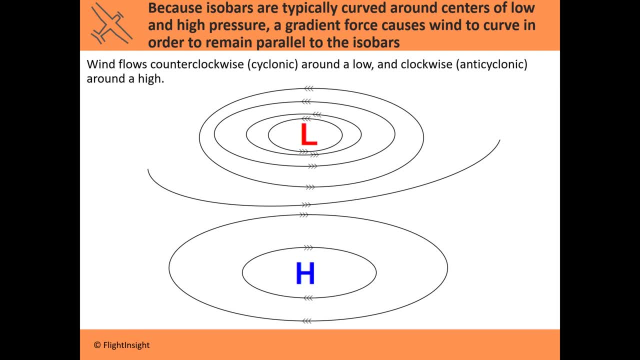 pressure to the right of wind. if we take these isobars and we turn them in on each other, right, they were parallel lines before and now we're curving them in on each other, which is the tendency that they have to do. you can see the 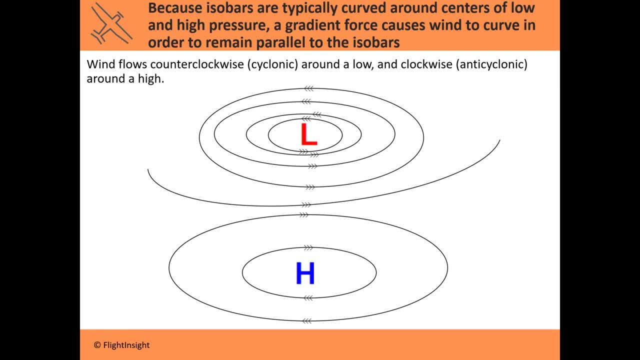 direction of travel of the air. in a low pressure system like the one I've got up top, Air is going to be flowing counterclockwise and you notice that as it does, that it stays consistent with that rule that the low pressure is always to the left of the wind, whether it's moving on the bottom or the top of 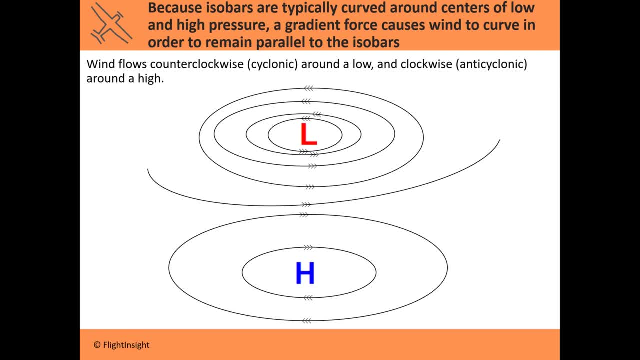 that oval as you're looking at it. And conversely, in the high pressure system you have clockwise rotation of air, keeping the high pressure to the right of that wind. In weather terms we talk about counterclockwise and clockwise motion as being cyclonic or anticyclonic. 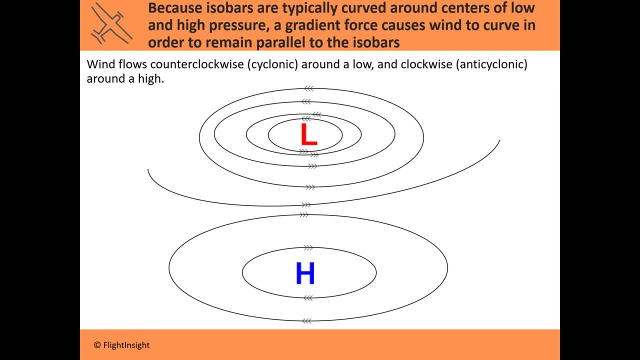 The way you can keep this straight in your head is that a cyclone is a low pressure system, a hurricane is a low pressure system. Those move counterclockwise in the northern hemisphere. So cyclonic activity is around a low pressure system counterclockwise, and anticyclonic is. 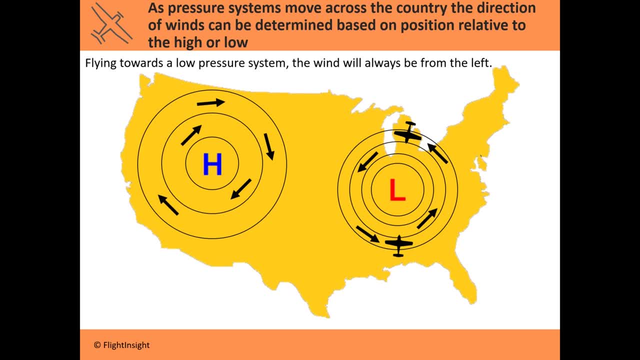 clockwise. Now that we know the direction of travel of wind in a high pressure, in a low pressure system, we can make an interesting observation is that as you fly towards the center of a low pressure system, you're going to perceive the winds from coming off of. 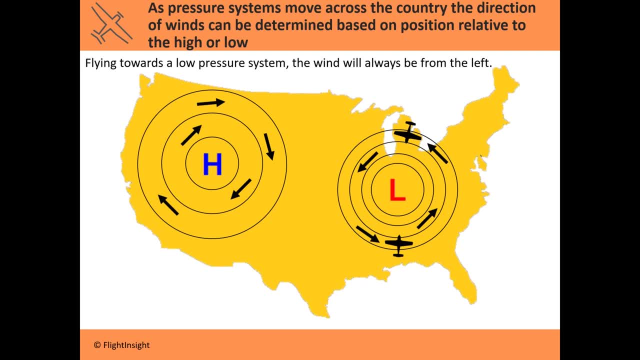 your left side and notice that that holds true whether you approach from the north the south, the east of the west of the system, because the winds are flowing counterclockwise in that low pressure system. if you're flying inbound, you're perceiving the wind off of your left side and, by that same token, if you fly, 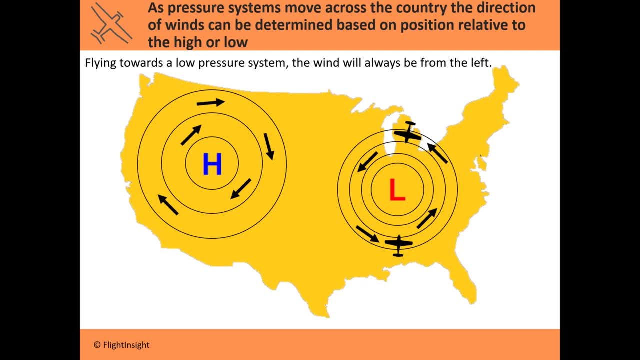 inbound towards a high pressure system. you're perceiving the winds to be off of your right side, regardless of how you're approaching- from north, south, east or west. so you can determine the type of winds that you would expect based on what you're flying into and, by the same token, if you know that you're flying. 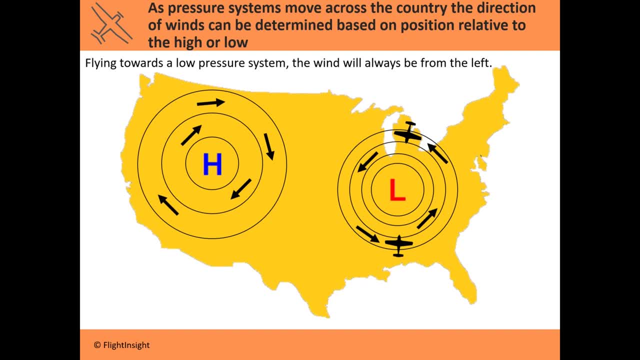 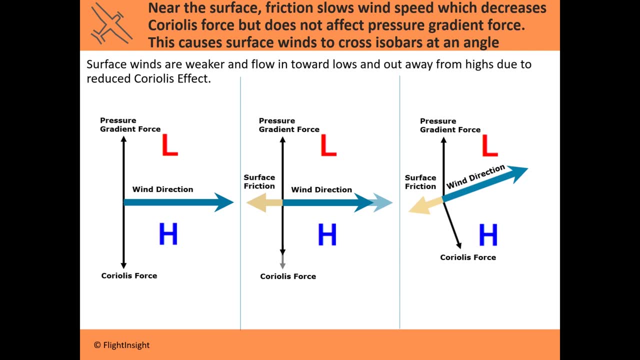 towards the center of a system, you can tell what that system is based on the direction of the wind. now there's one more complication to this. so we talked about the pressure gradient force, we talked about that initiating force, what causes the wind to start blowing, and we talked about 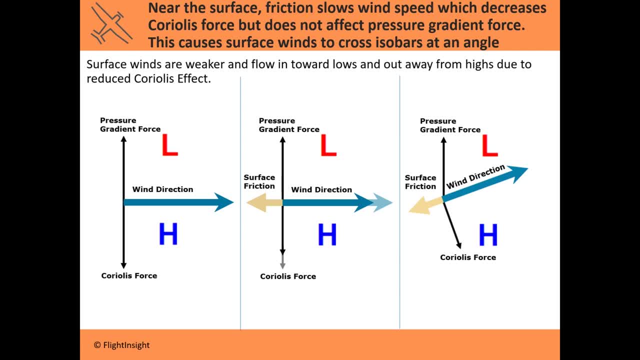 Coriolis force. what causes the wind to curve? there's another complicating factor here, and that's the fact that as you get close to the surface, the air that moves across it is going to be deflected or it's going to be affected by that wind. 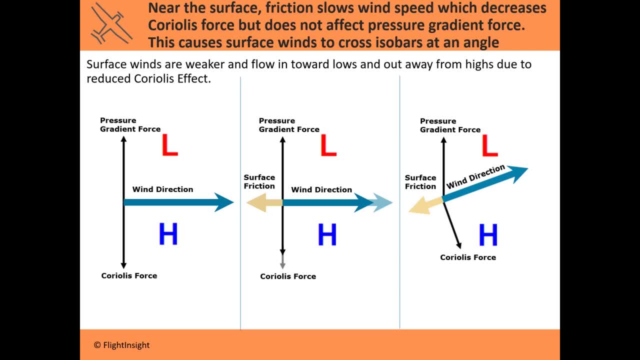 the pressure gradient doesn't change whether you're talking about being close to the surface or high up above the surface. it's just a function of how different are the pressure systems and how close together are there. but what does get affected is the Coriolis force. as you get close to the surface, the friction that slows down. 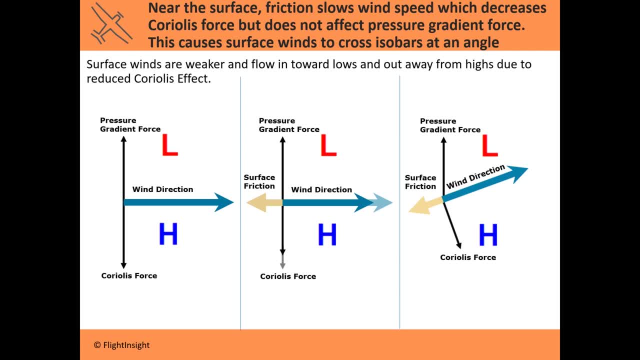 moving air because of things like trees or buildings or rugged terrain or anything jagged on the surface of the earth that gets in the way or that slows down that Coriolis force. it's going to have another veering effect on the wind. so if we start with that simple model from a few slides ago, we take kind. 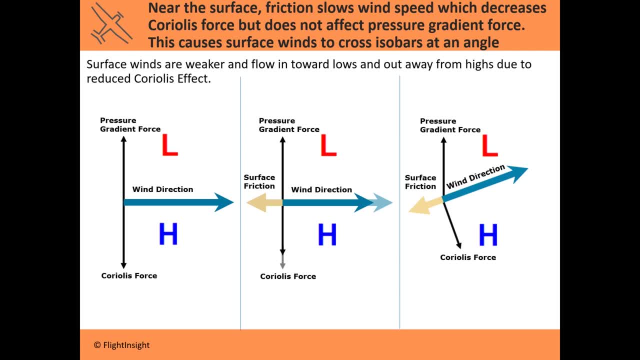 of the end state of the pressure, gradient, frequent, and we take a moment gradient force and the Coriolis force in that first third of the slide here where you have counterbalancing pressure, gradient force and Coriolis force which causes a wind direction. 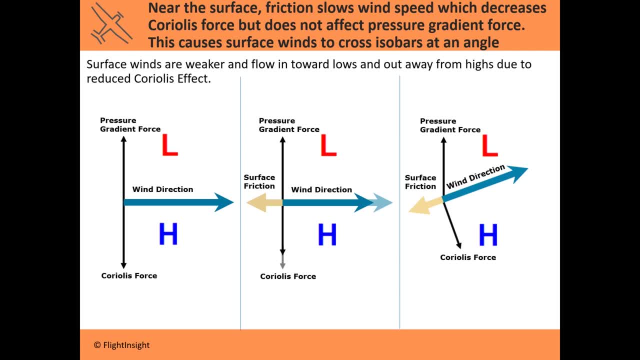 which goes exactly parallel with an isobar. In other words, it splits right down the middle between a low pressure and high pressure system. Well now, if you add surface friction, you're slowing the wind down. You're not slowing the force of the wind down, but you're slowing the 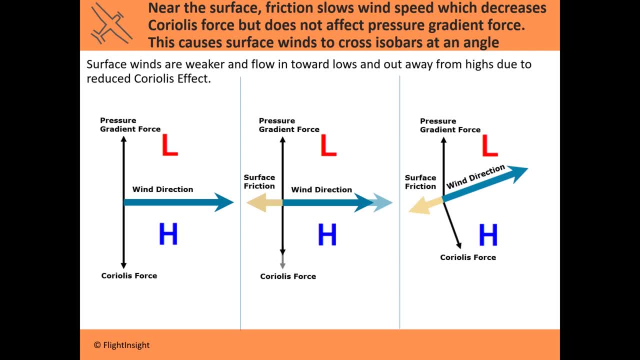 actual wind speed down. If the wind speed goes slower, as you see in that second half or that second third of the slide, that means that the Coriolis effect isn't going to have as great of an effect on the wind right. The faster the wind flies, the more the spinning of the earth is going. 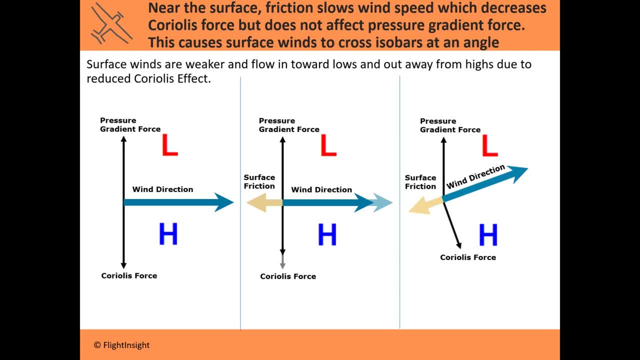 to cause it to deflect. So a slower wind speed means a smaller Coriolis force. A smaller Coriolis force means the pressure gradient starts to win out again. So that's going to cause the wind to change direction, that it's going to veer again and 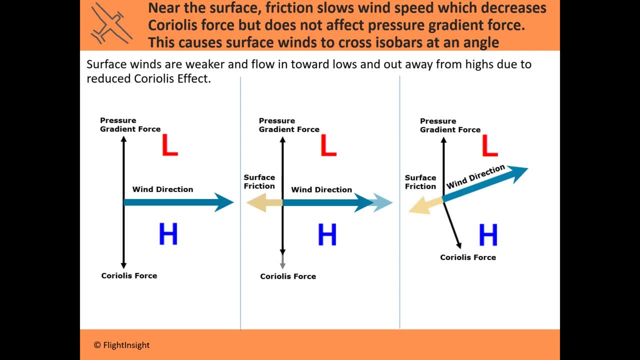 it's going to veer away from a high pressure system and it's going to veer inwards towards a low pressure system. So these are the three factors into how fast is the wind blowing and what direction is the wind going to come from. And you see it all right there in that third. 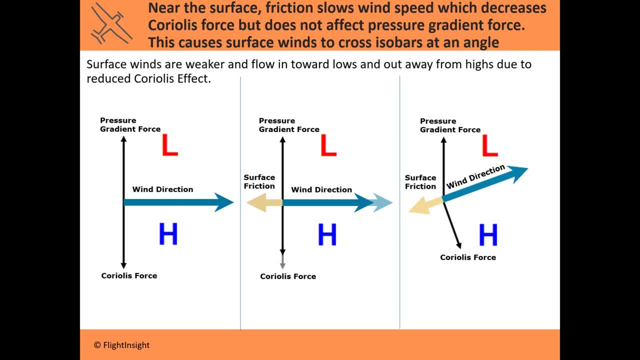 panel of this slide here. It's pressure gradient force that causes the wind to blow. it's Coriolis force which causes the wind to veer, surface friction which slows down or retards the Coriolis force. Those are the three forces which. 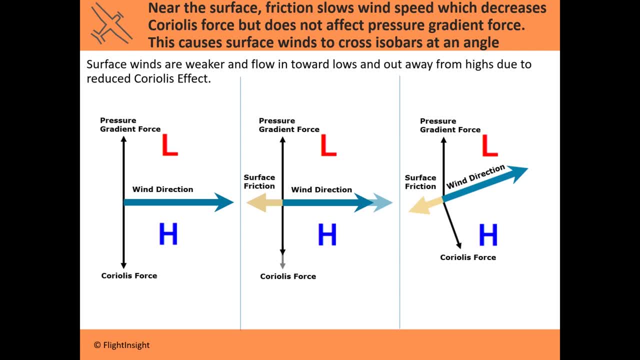 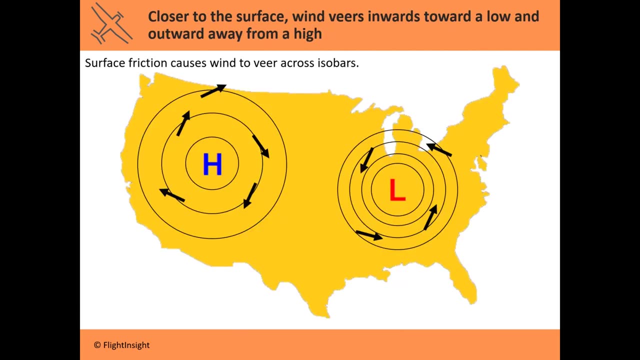 determine wind speed and direction, And when they're all used in balance like this, what you have is wind that's off a little bit of skew and it skews away from a high pressure system and towards a low pressure system. Here's what that looks like on our pressure map. So again, you have